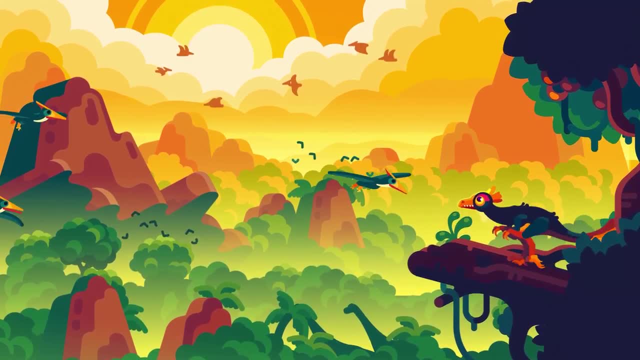 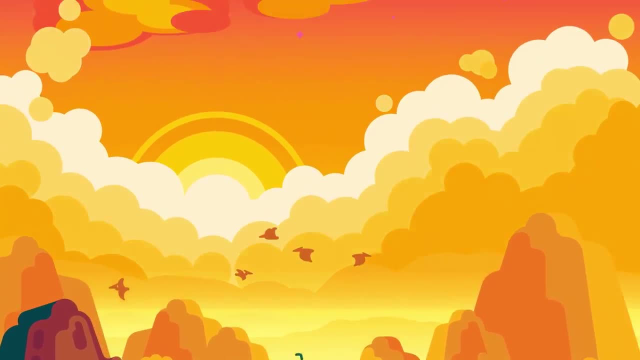 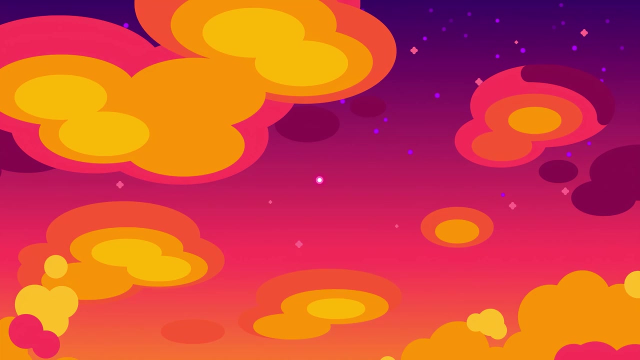 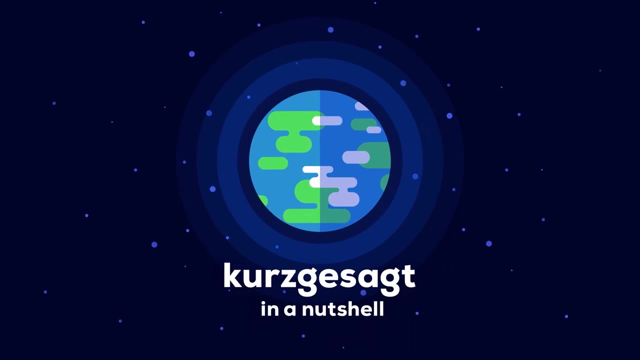 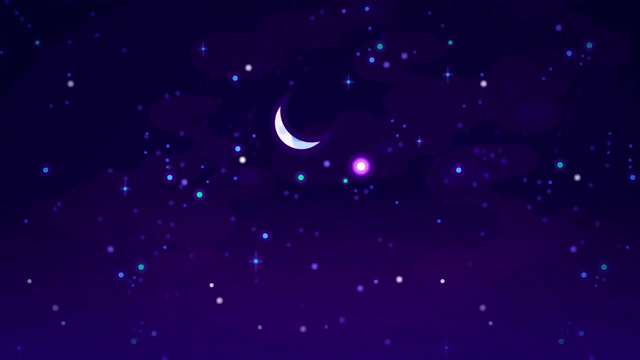 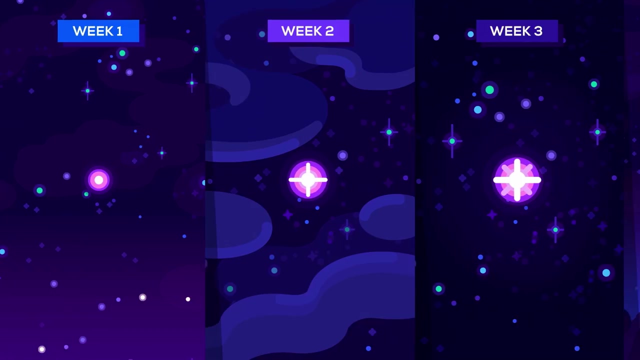 In some countries, as if five million years ago, Thirty six million years ago – maybe on a Tuesday stars one night they may have noticed the appearance of a new star, a tiny dot that for many weeks slowly became bigger and brighter, Until one fateful day it looked like another. 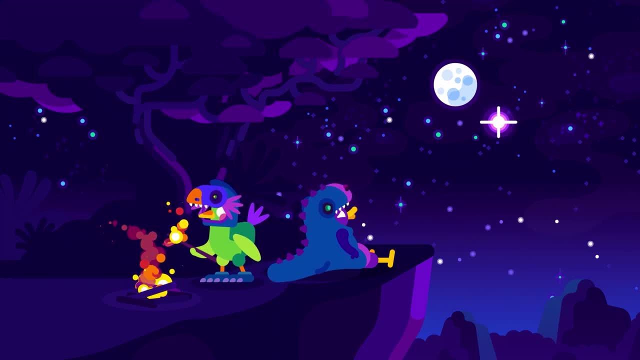 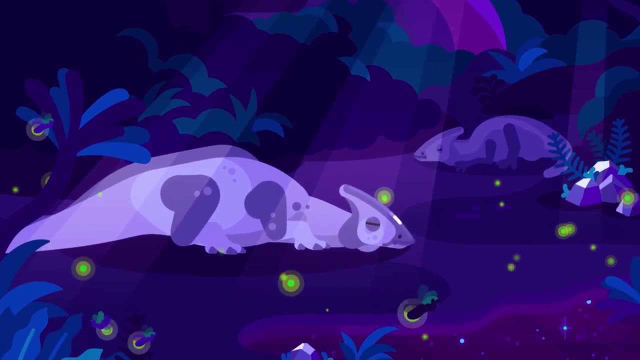 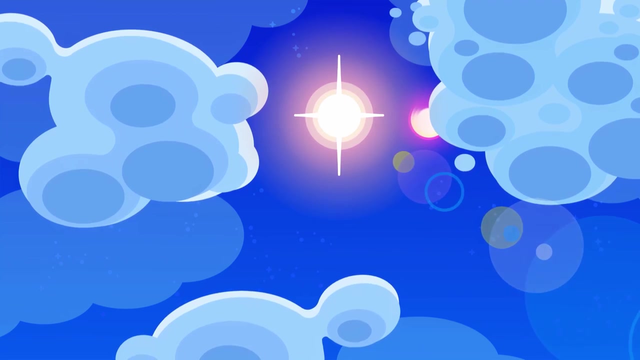 small moon in the night sky, And then it faded from sight as it dipped into Earth's shadow. For a few more hours, the illusion of continuity was upheld, Until it was not anymore In the morning. the object suddenly appears again, Now almost as large as the sun in the 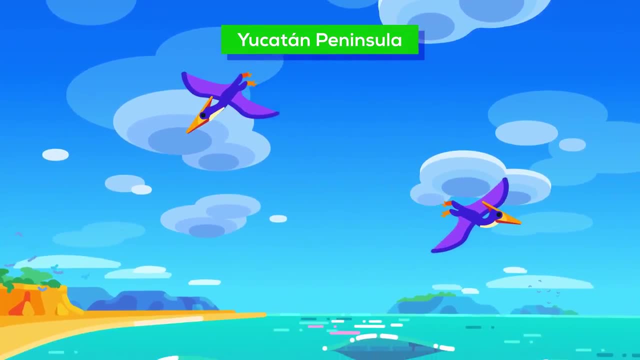 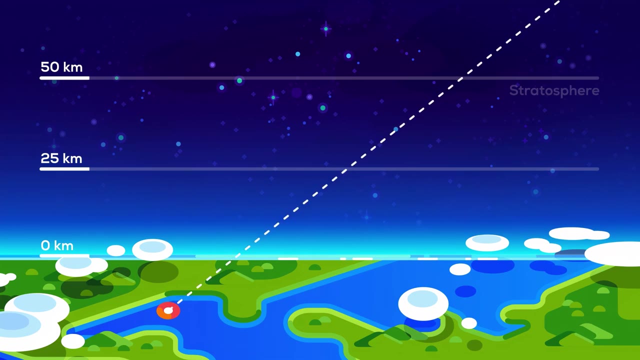 sky and growing every moment. heading for the coast near the Yucatan Peninsula, It takes the asteroid only seconds to pass through the thin layer between space and the ground, to make contact as it enters the atmosphere at almost 60 times the speed of sound. 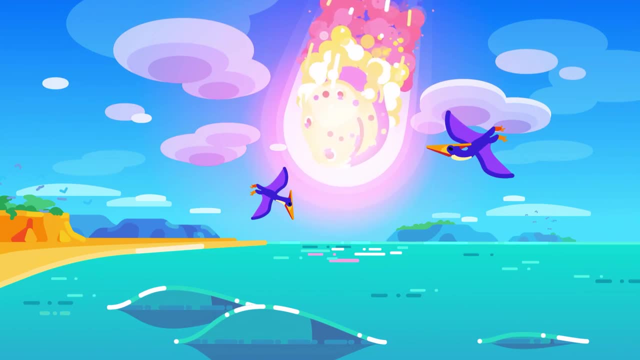 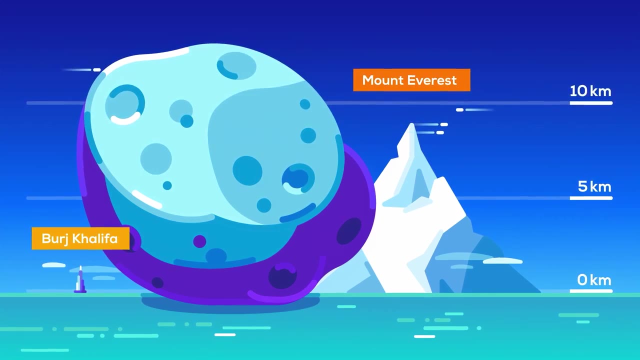 Let's stop time. Here we see the unnamed asteroid about to commit speciesism. The asteroid is located on the far side of Mount Everest, on the far side of the Pacific Ocean. It is located on the far side of Mount Everest, on the far side of Mount Everest, on the far side of. 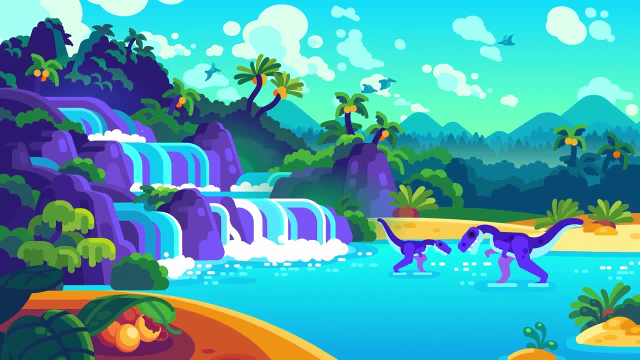 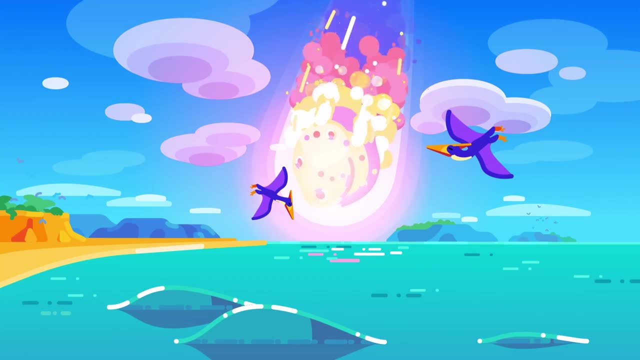 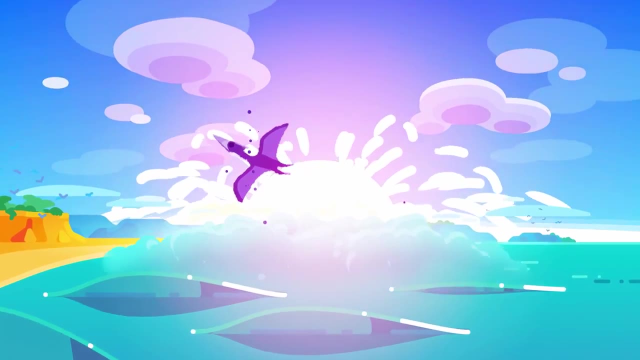 the Pacific Ocean. At this moment, the world was one way In a fraction of a second, it would be fundamentally different. Let's make the transition. As the asteroid hits the shallow ocean and the bedrock below, the energy of billions of nuclear weapons is released all at once as the asteroid. 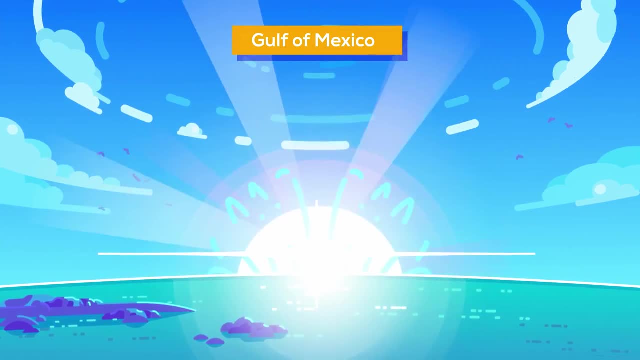 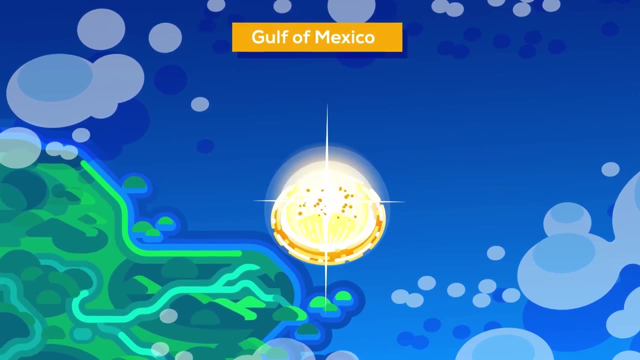 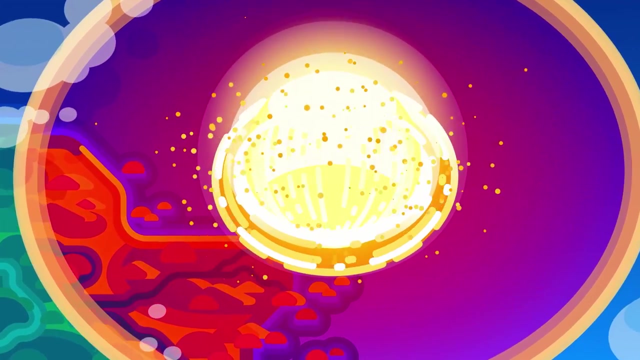 vaporizes. A flash of light illuminates the sky as an eerie bright white sphere grows over the Gulf of Mexico. Bedrock melts into seething hot plasma at tens of thousands of degrees Celsius. The thermal radiation from the explosion travels at the speed of light and immediately burns. 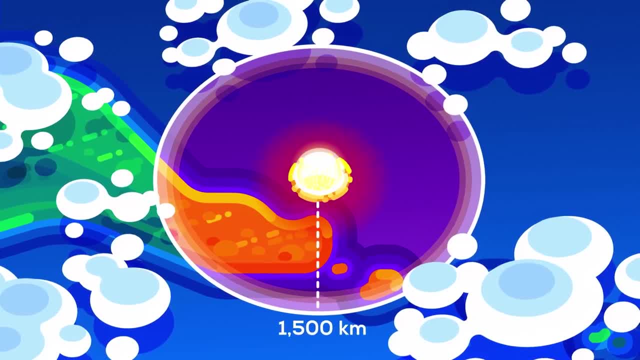 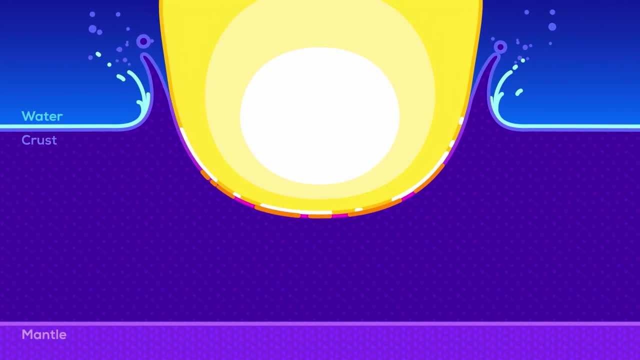 everything within a radius of about 1,500 kilometers, while the energy from the impact pushes so hard against Earth's crust that it loses all strength and flows away from the impact site like a liquid, creating a hole 25 kilometers deep and 100 kilometers wide. 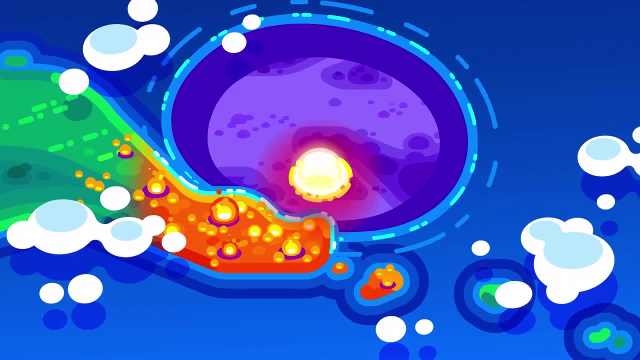 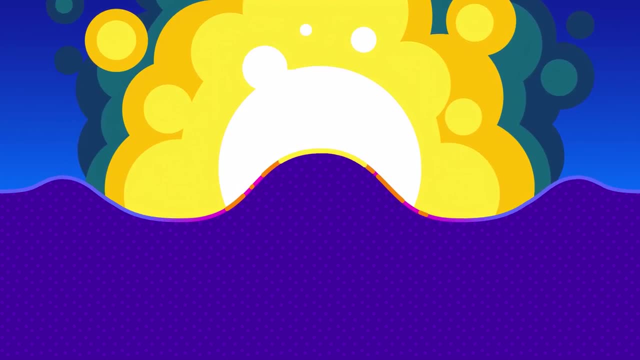 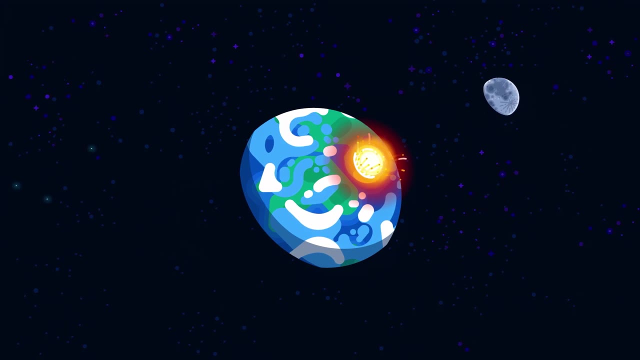 The ocean is pushed back for hundreds of kilometers, like when a kid jumps into a puddle. As the crust bounces back, melted and flowing crust forms a temporary mountain stretching 10 kilometers into the sky. An incredible amount of material is blasted into the higher atmosphere. 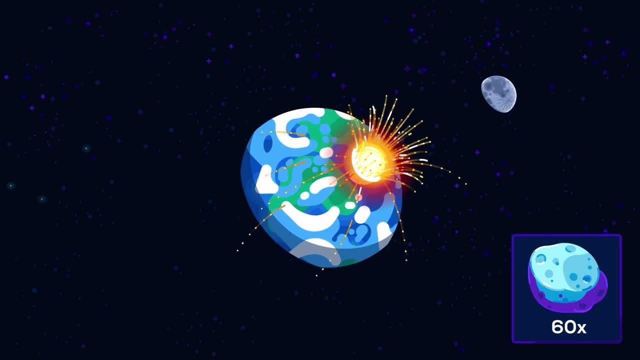 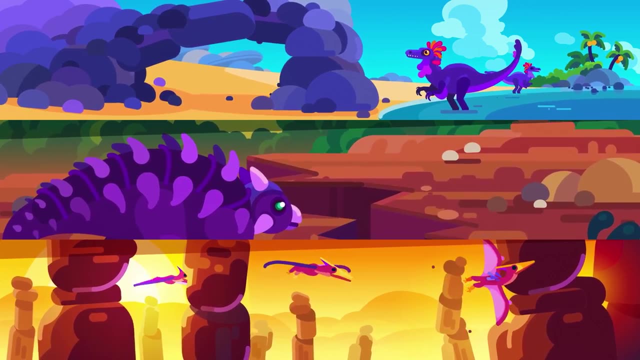 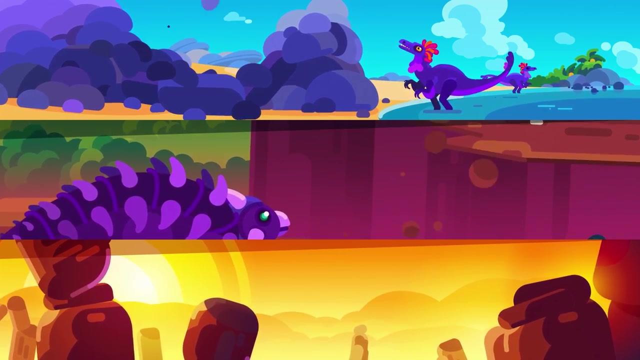 or even out into space, as much as 60 times the original mass of the atmosphere. The violent of the strike is felt everywhere on Earth within minutes. A magnitude 11 earthquake may be the most powerful quake any living thing has ever witnessed in billions of years. It is so insanely strong that in India it might have shaken gigantic. 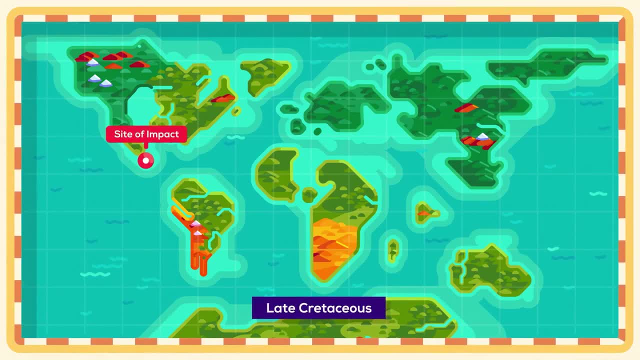 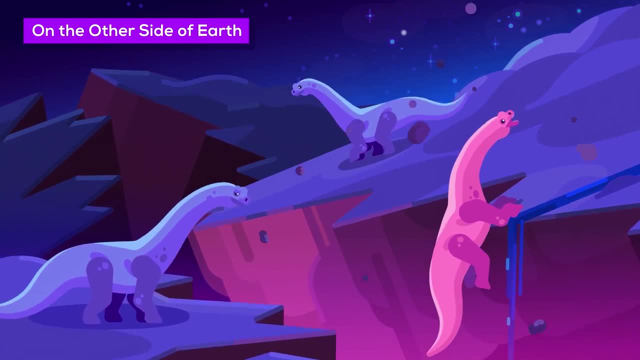 lava fields and causes volcanic eruptions that would last for 30,000 years and cover half of the Indian subcontinent with lava. Even on the side of Earth, opposite the impact, the ground still moved by several meters. Nobody would sleep through this day. 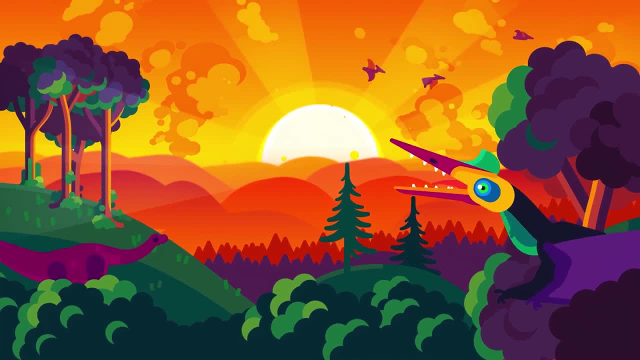 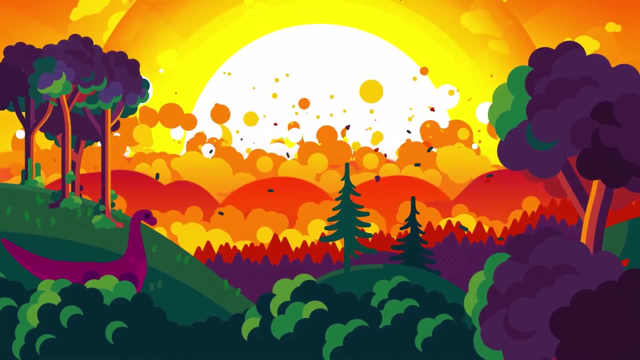 The gigantic explosion crashes against the atmosphere with unprecedented violence and causes a shockwave that reaches speeds of more than 1,000 kilometers per hour near the site of impact, similar to the hyper-hurricanes on gas giants like Neptune In middle America. 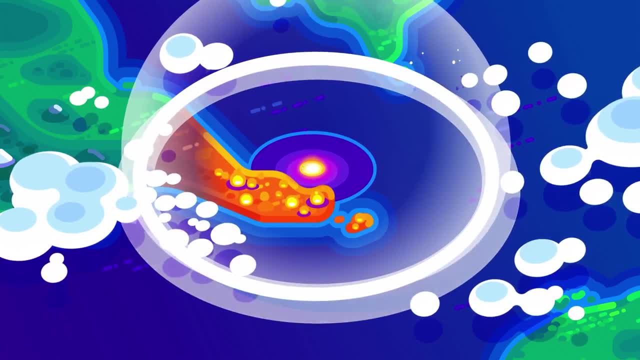 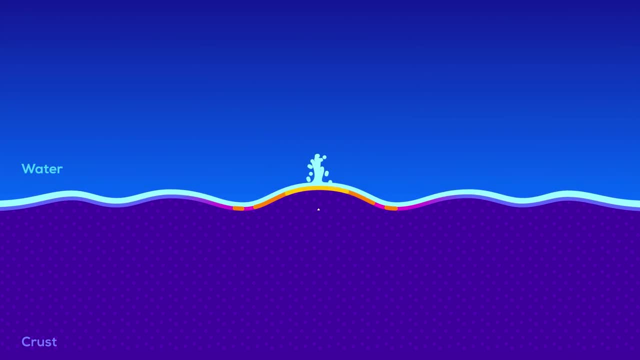 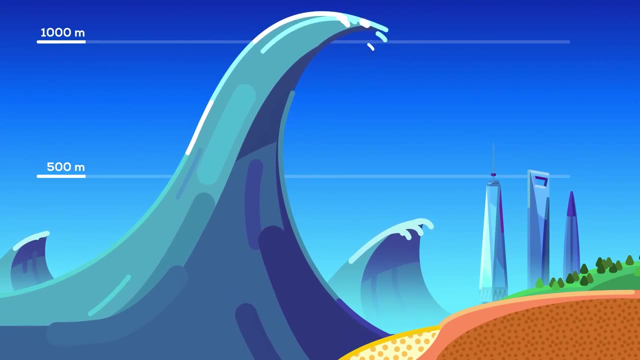 basically any soil, vegetation or animal is just shredded into pieces and catapulted thousands of away. Now the previously displaced oceans return. As the temporary mountain at the site of impact collapses, a ring of tsunamis as high as one kilometer, enough to cover all skyscrapers. 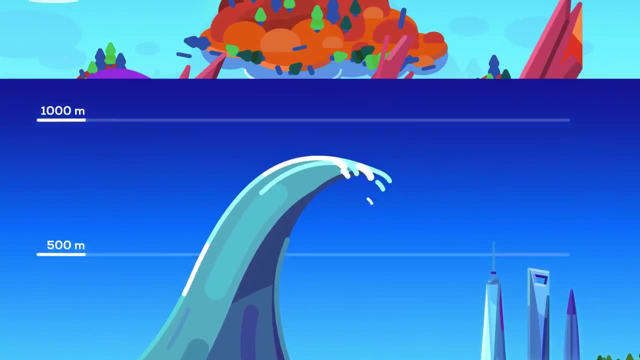 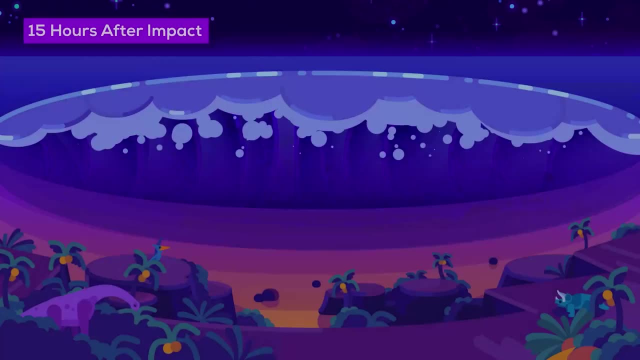 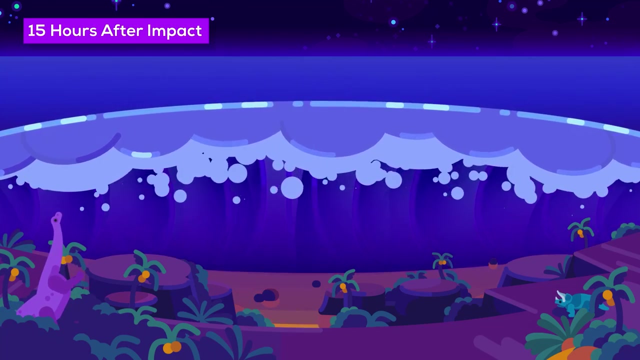 humans would ever build heads in all directions As they crash into the coasts of the continents surrounding the impact: they will drown thousands of kilometers of coastline. Fifteen hours later, some of the waves that get refracted around South America will still tower as much as 100 meters into the sky. But we still haven't talked about the worst. 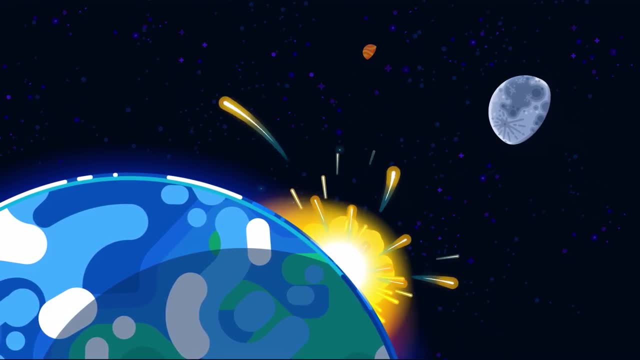 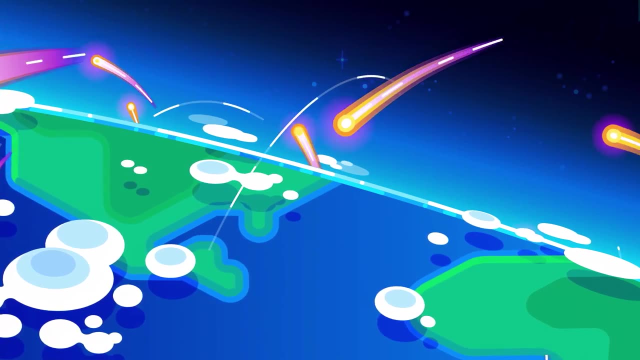 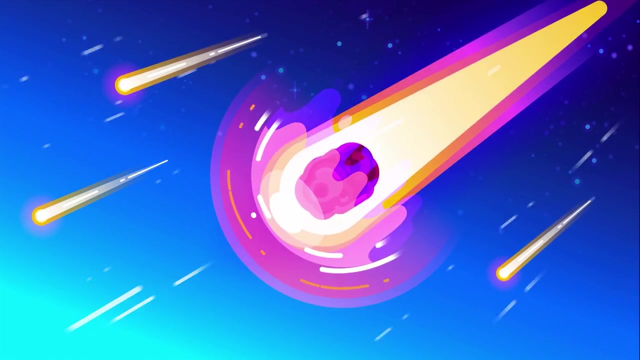 thing. yet A lot of the debris yeeted into space will orbit Earth for thousands of years. Some may hit the Moon or even Mars, But most of it comes right back. When things fall through the atmosphere at such speeds they get very hot, As in hundreds of degrees hot, And this happens to millions of 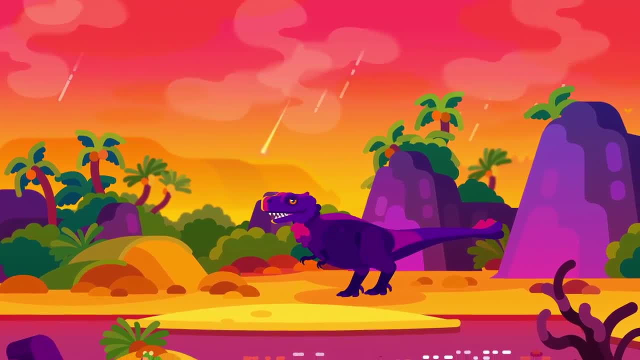 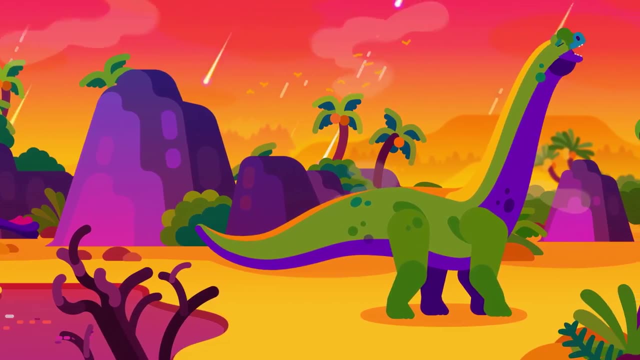 tons of material everywhere. This rapidly heats up the atmosphere to insane temperatures. We don't know exactly how hot it got or how long this heat shock lasted, but there are two ideas here. Either the air was heated to hundreds of degrees for a few minutes. 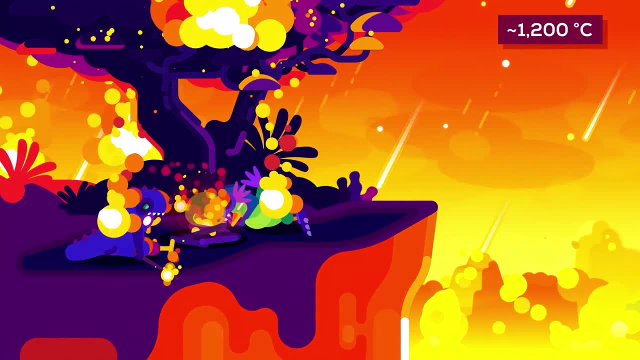 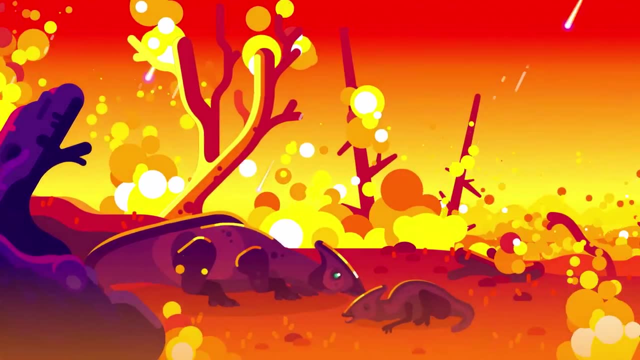 or to thousands of degrees for around one minute. In any case, the air became as hot as the inside of an industrial oven. How bad the global effects of this were is contested, but if enough heat reached the surface, a lot of plants and animals would have died very quickly if they couldn't. 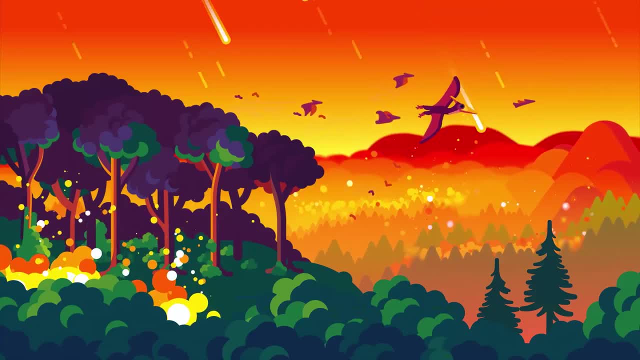 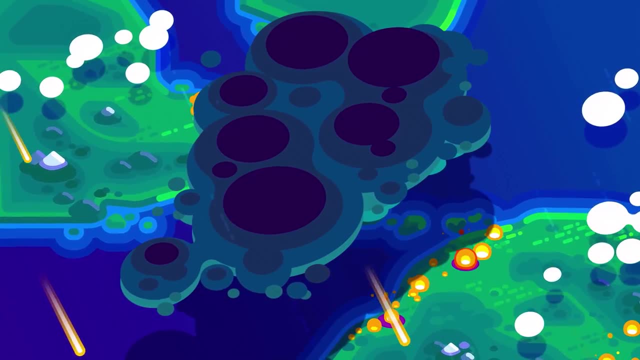 bury themselves or escape from the heat, And that's what we're going to talk about in this video. So let's get started. The heat, together with raining debris also, may have ignited material on forest floors and sparked wildfires as the Earth rotated under the searing hot blue In a few hours. 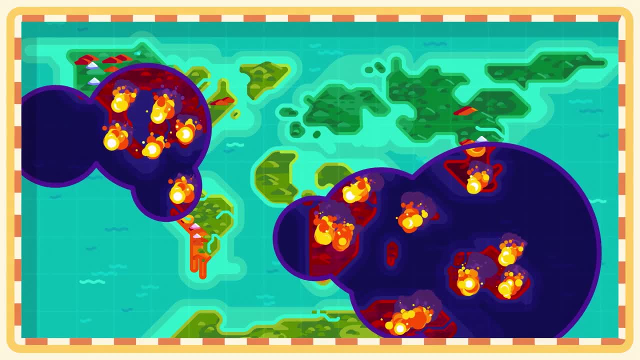 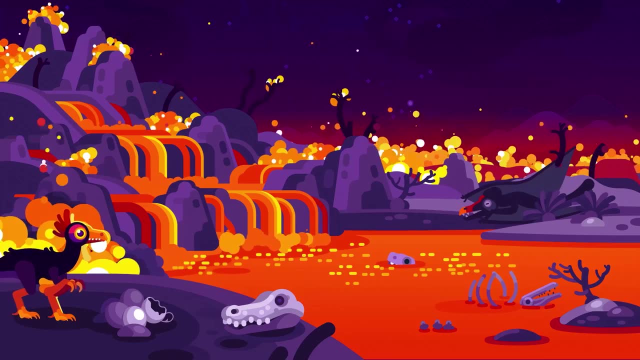 massive wildfires were probably burning around the globe. Some of them may have lasted for months and turned Earth into a horrifying, hot, hellish version of itself. As the day of the impact draws to an end, many of the dinosaurs are already dead. 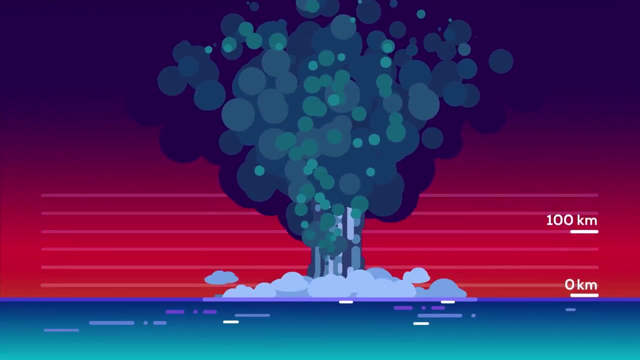 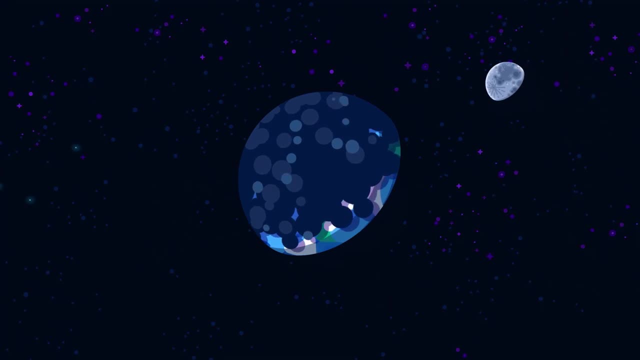 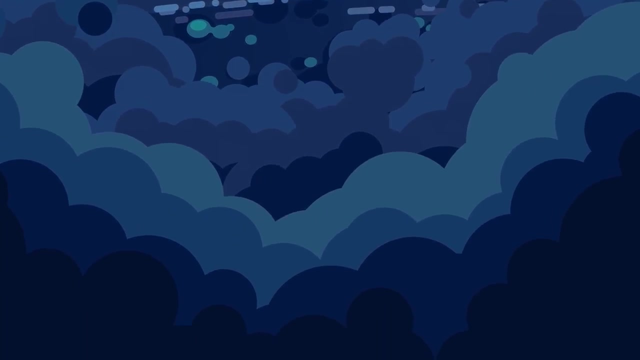 but the worst is still to come. The gigantic plume of vaporized material reaches the upper atmosphere and spreads around the whole globe. Together with the soot from the burning planet and the aerosols generated at impact, the planet sinks into a deep darkness. 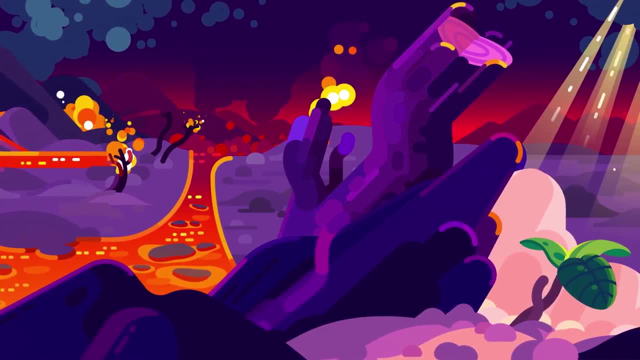 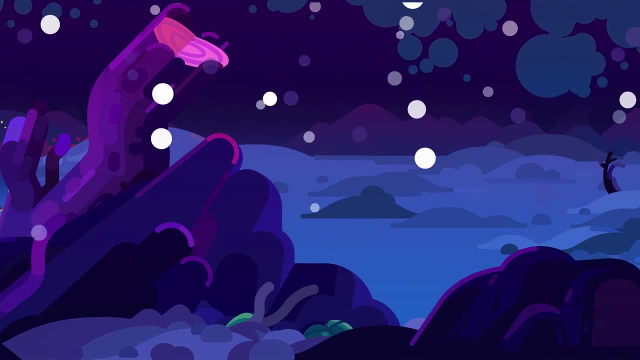 with only the remaining raging fires illuminating the scenery. Whatever plants survived the firestorms will now be starved for sunlight as global photosynthesis is temporarily shut down. Within days, temperatures will drop to about 20 degrees Celsius, and the temperature will drop to about 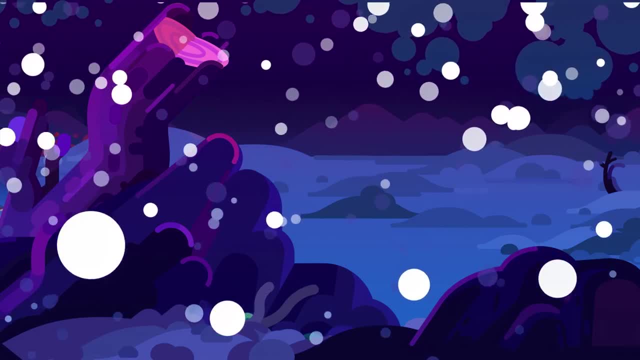 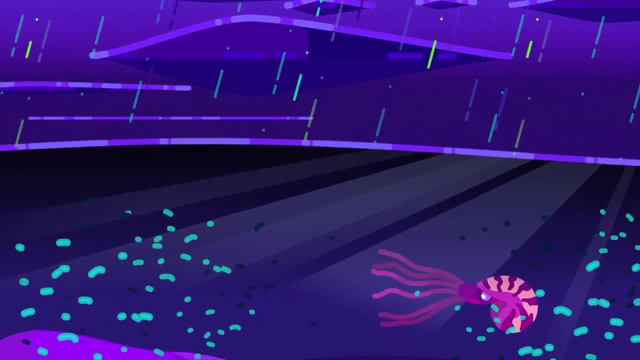 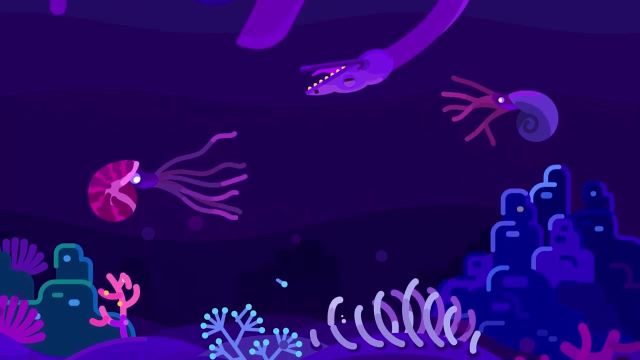 25 degrees Celsius. The oceans were especially hard hit. The lack of sunlight killed over 90% of plankton, which formed the basis of the food web of marine life. Ultimately, this would kill off the large marine reptiles and ammonites that used to dominate the seas, The biosphere that 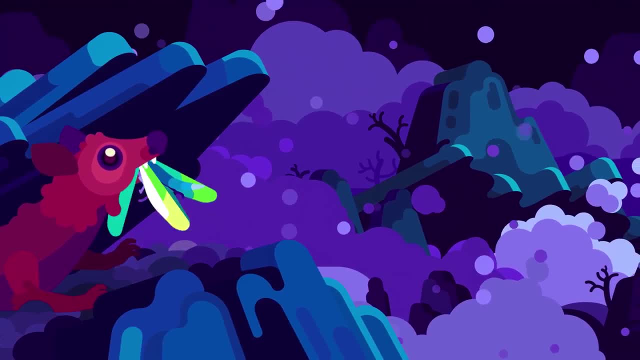 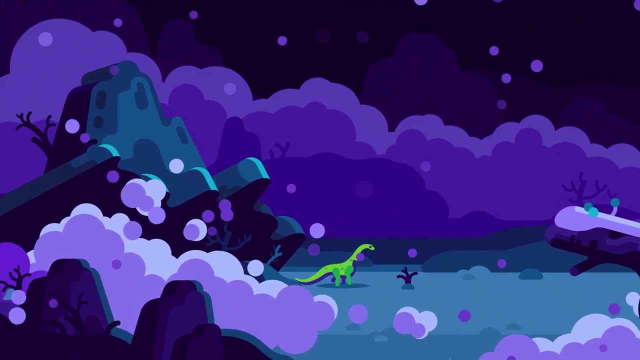 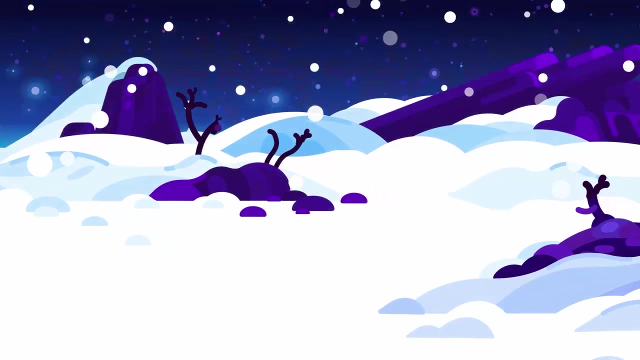 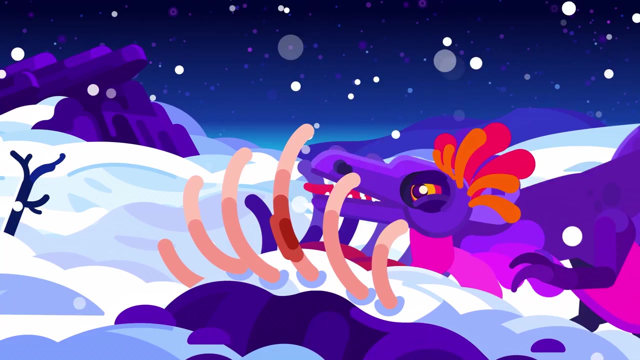 survivors now find themselves in is like an alien landscape. Ash, debris and the burned remains of the formerly lush and blooming life will soon disappear and the environment will become a mess. The planet will be a hostile and deadly place. The sudden global winter will last for 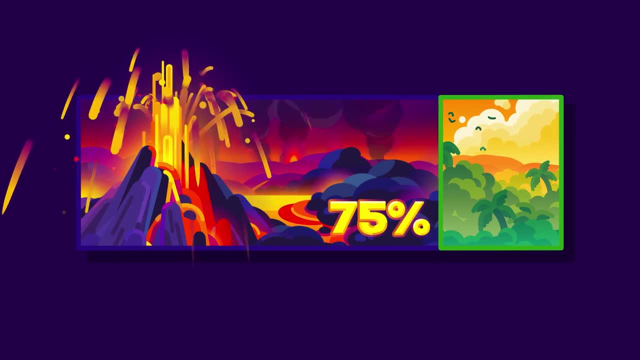 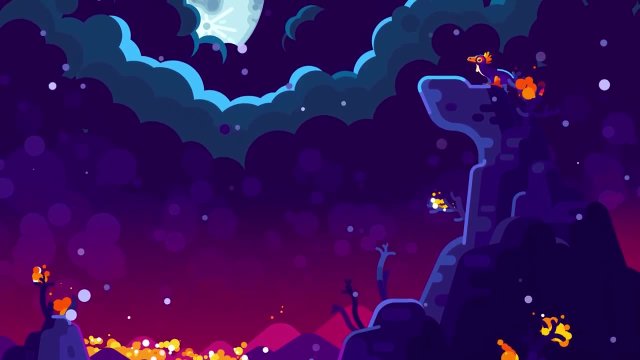 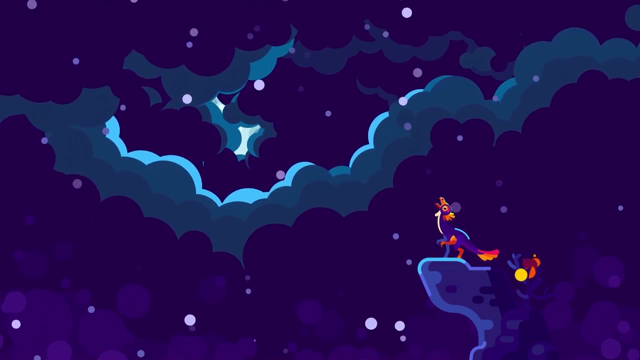 decades, At least 75% of all species on Earth will just vanish from existence, And so, as the day ends, the world is suddenly different. The continuity that went on for millions of years is no more. The era of the dinosaurs is over, Just like that. 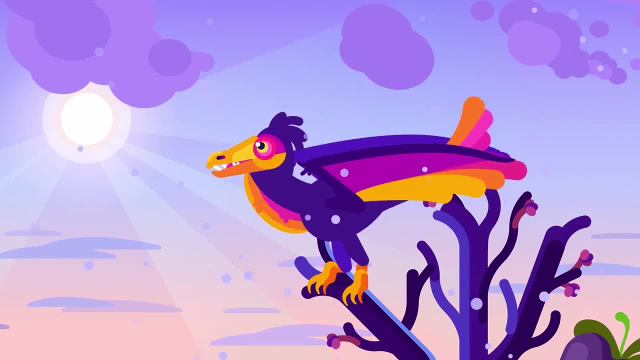 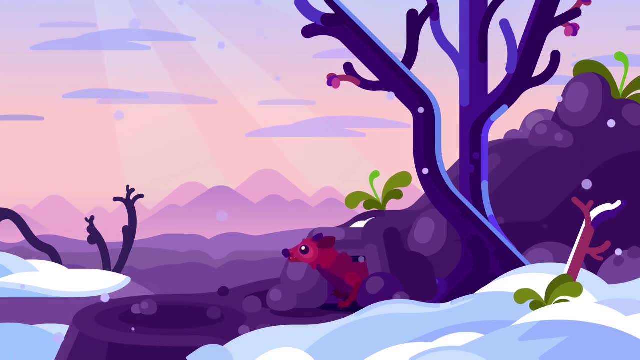 Eventually, from the ashes of the old world survivors emerged Birds that are the direct descendants of the dinosaurs and mammals that would eventually become the dominant animals on the planet. Without the asteroid, who knows what life on Earth would look like today? 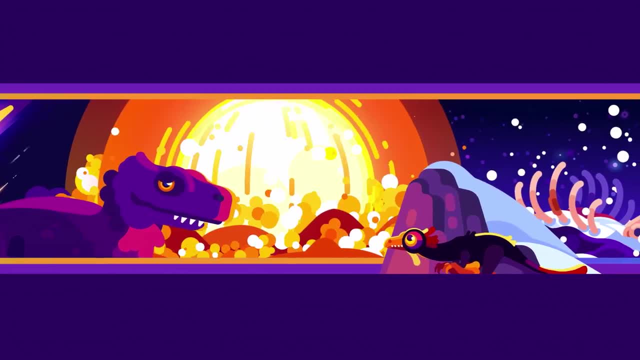 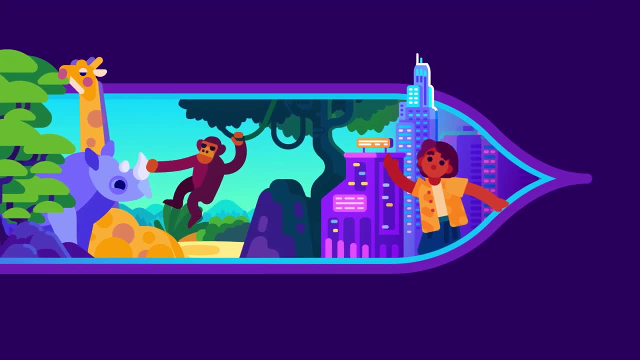 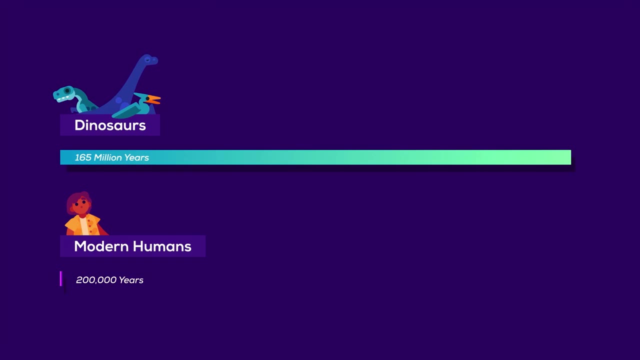 Without the sudden disruption of dinosaur continuity that completely changed the planet and all life on it, we might have never had the opportunity to become what we are today. It's not clear how long the human era will last. So far, modern humans have been around for 0.1%. 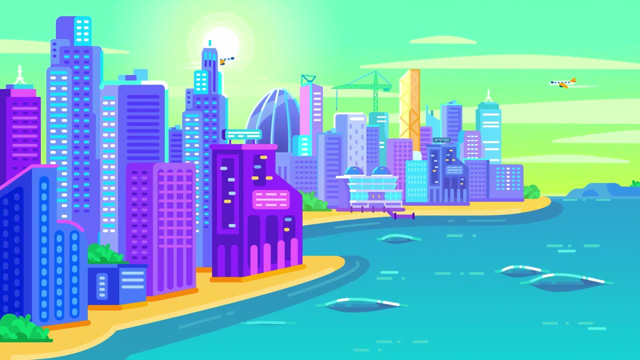 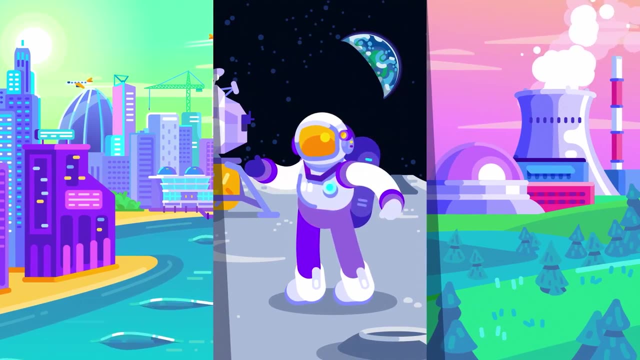 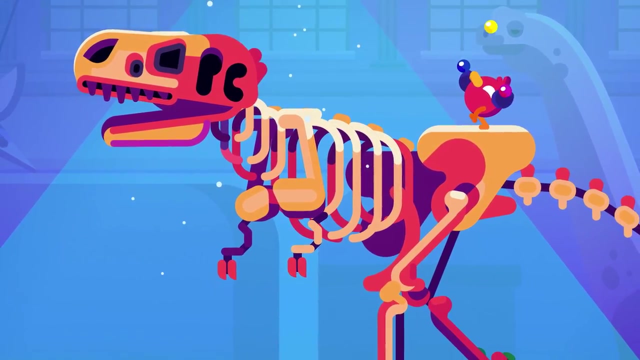 of the time the dinosaurs were, And in this short amount of time we've achieved impressive feats, from making the world our own to reaching space and splitting the atom. Yet our future and our long-term survival are not a given. If we're not careful, it could end in an instant like the age. 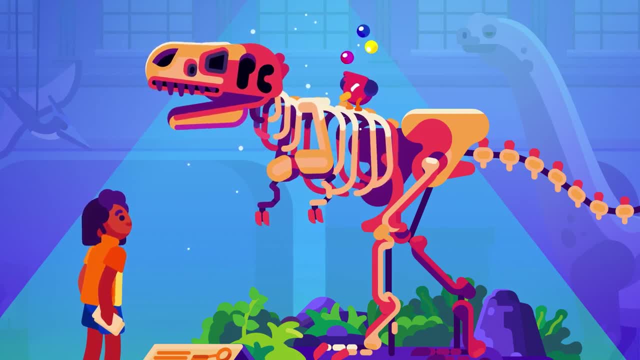 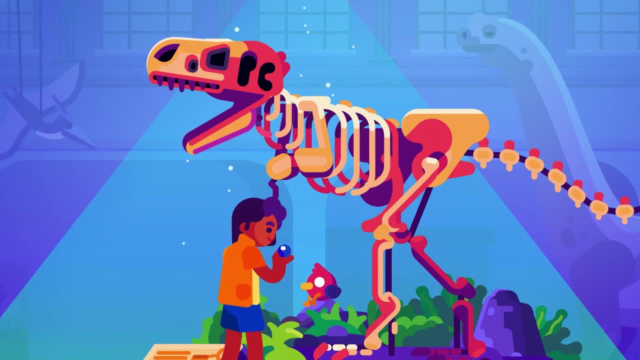 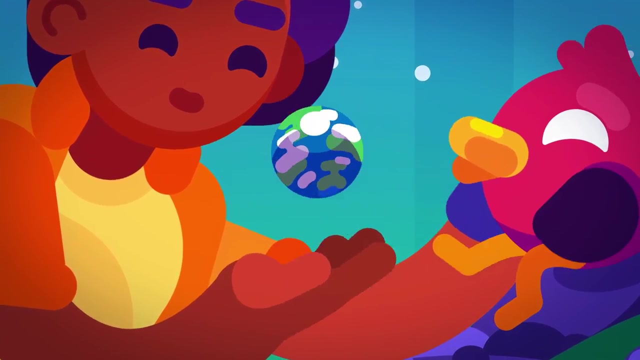 of the dinosaurs ended, But, in contrast to them, we know that our continuity is fragile. even if it doesn't feel like it, We can be prepared and be vigilant and hopeful. If we're lucky, our journey will go on for a long, long time. Speaking of journeys, we want to address something 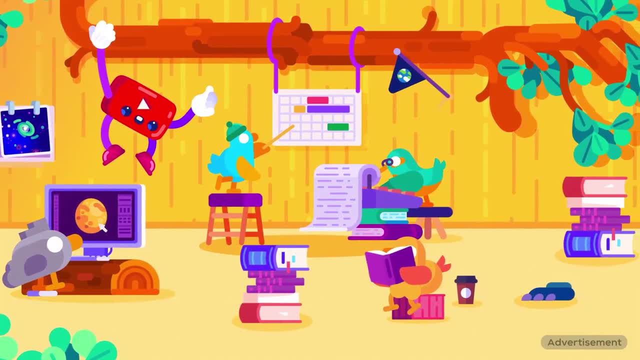 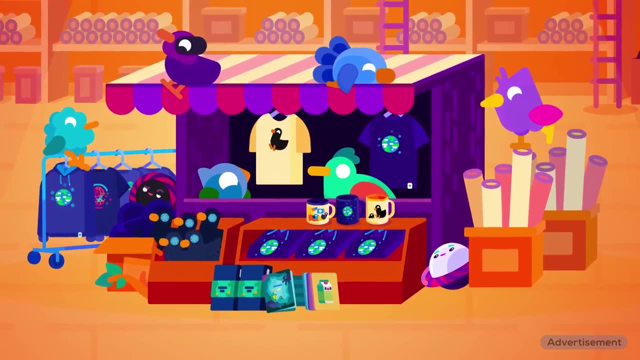 in the spirit of transparency. Kurzgesagt has changed in the last two years. We've become more than a YouTube channel or animation studio, and now also run a paper shop that sells hundreds of thousands of calendars, posters and notebooks. That's not a happy accident. many of us have a 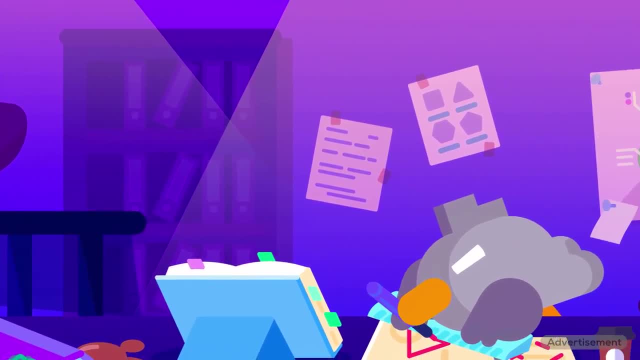 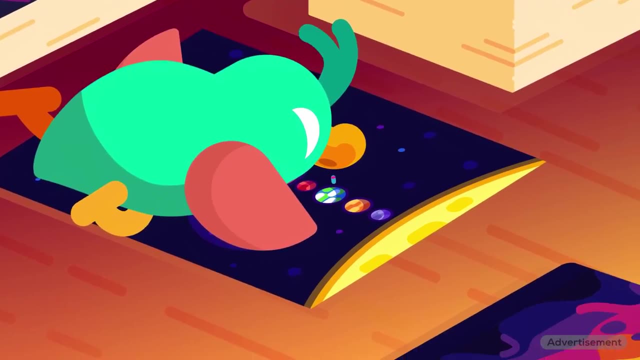 background in graphic design. Paper products are our roots and we actually started out creating posters, books and print infographics. We love that. you can touch them, smell them, nerd about small details and printing techniques. That's why we're here today. We're here because we want to. 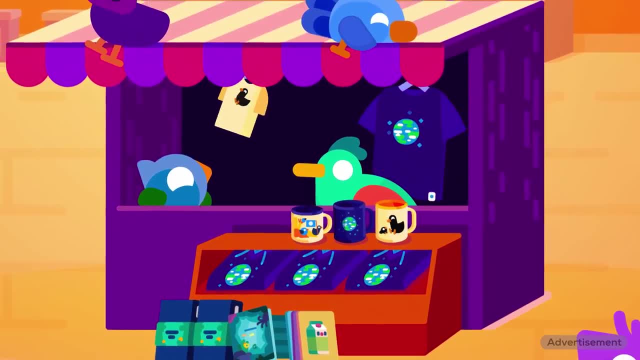 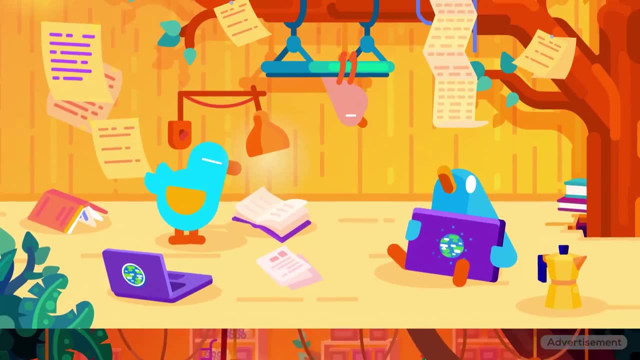 help you. Just like the channel. we started small and without great ambition. Step by step, we found the right printers and papers, learned about shipping and expanded our shop. We put a huge amount of research, love and hours into it, because this is the only way we know how to do. 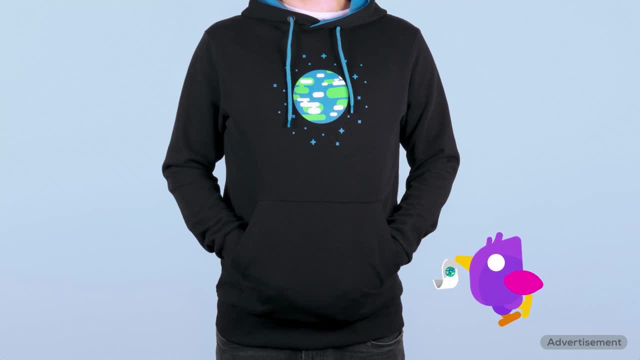 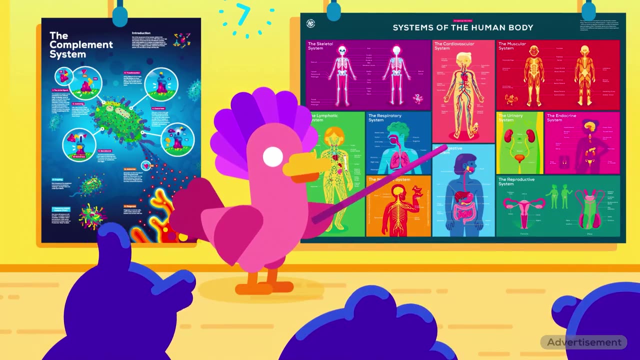 things. We don't just want to make generic merch. we want to make things that fit our mission of making science exciting and creating beautiful things, Things that persist and are made with high quality and love. Our shop gives us the opportunity to create things that we love. 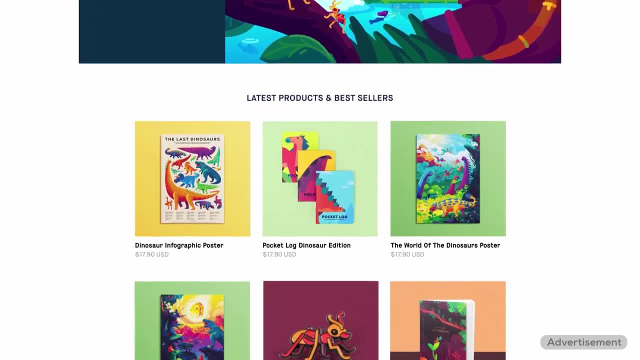 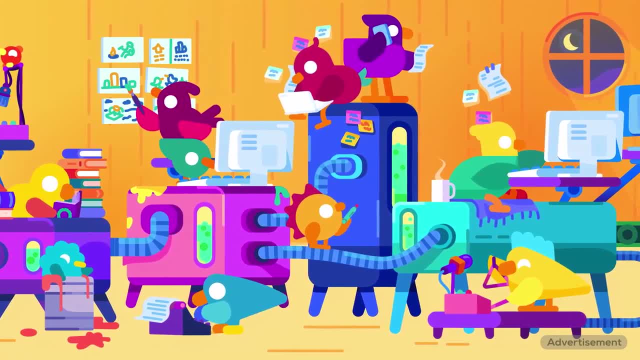 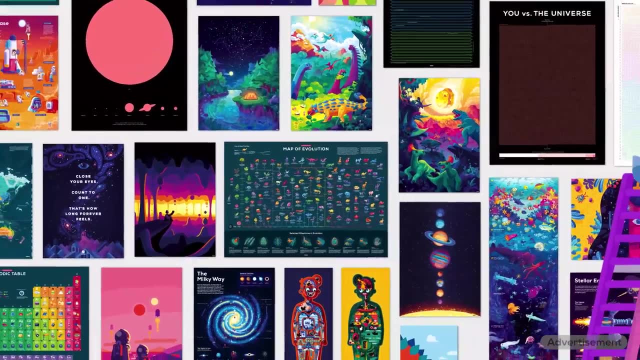 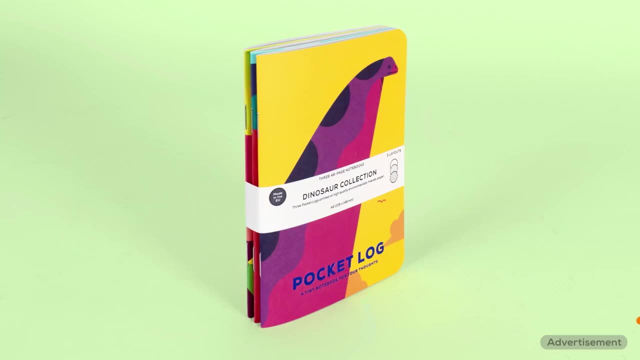 for everything we do on this channel, which also keeps us independent and our videos free for everyone. So we want to build further on that and create more things that last. We've just started a new notebook line called PocketLog that we'll expand on in the future. The first edition is a 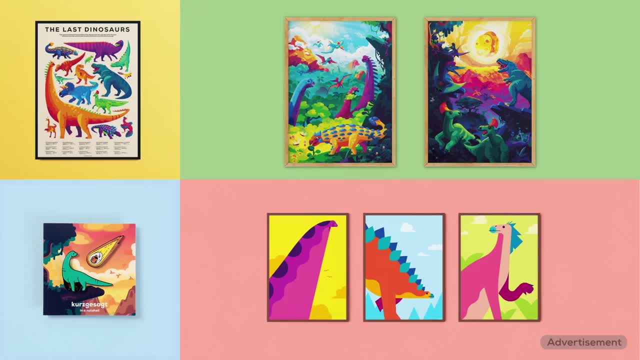 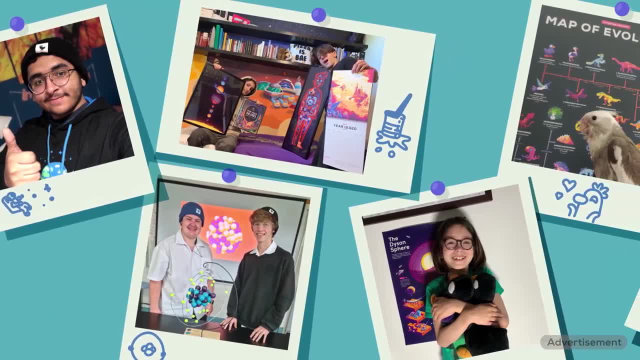 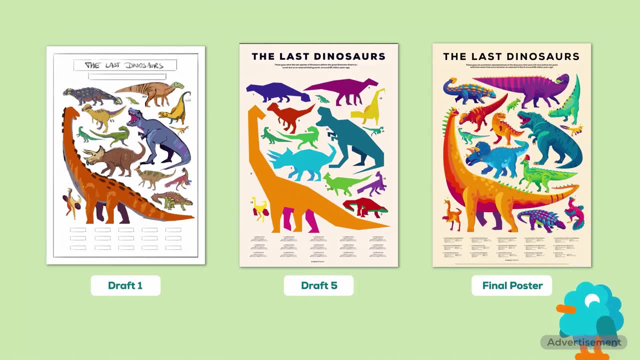 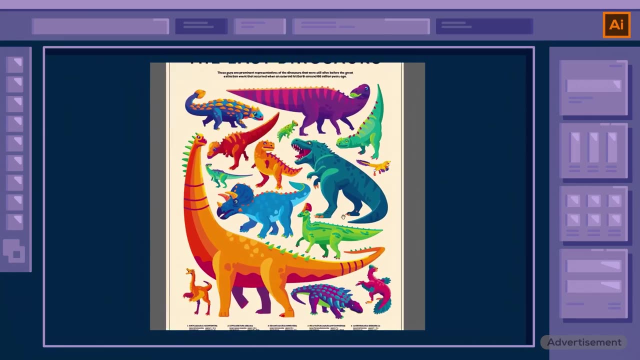 published articles like all this soon. Please continue your work at PocketLog. Your first Exhale will lead to a fantastic page about how important it is to make in-step print-free magazines in the now unpreserved world of of science. Our products havesche któtg to introduce each year time to regarding the future of all science. 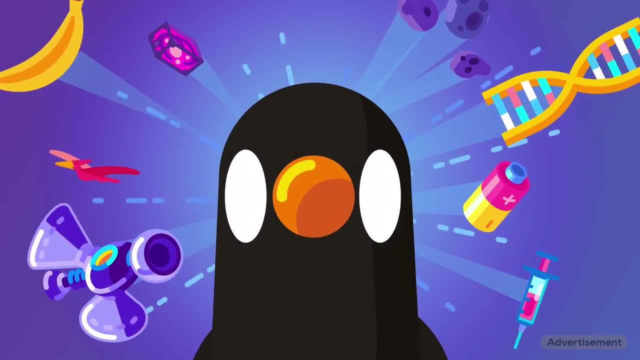 and make something from it, expert piece to exercise right now into the future of science. The books and design offers will do not only provide the tools for peace of mind, objectives for future SmartToGo to use in future state, opportunity for delivery by stateから. and that's already. 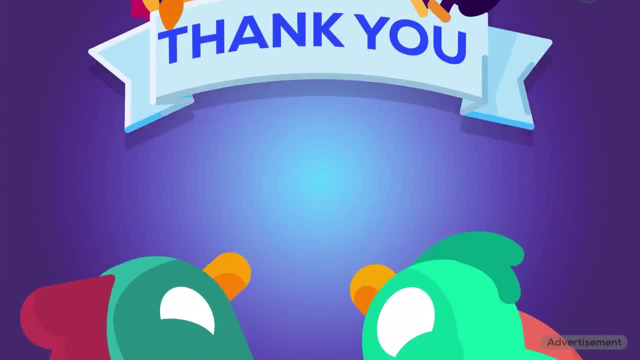 much needed. We're looking forward to making fun sciency stuff for you, no matter if it's a video, a poster or something else entirely. Passion didn't share them since Poster measure until 14 July. Thank you for watching. 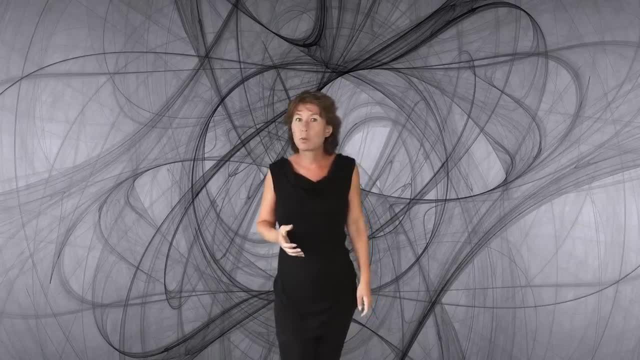 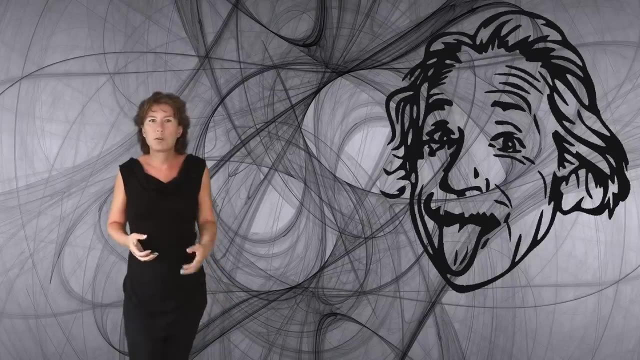 Today I want to explain how we know that the way Einstein thought about gravity cannot be correct. Einstein's idea was that gravity is not a force, but it is really an effect caused by the curvature of space and time. Matter curves spacetime in its vicinity and this curvature in return.